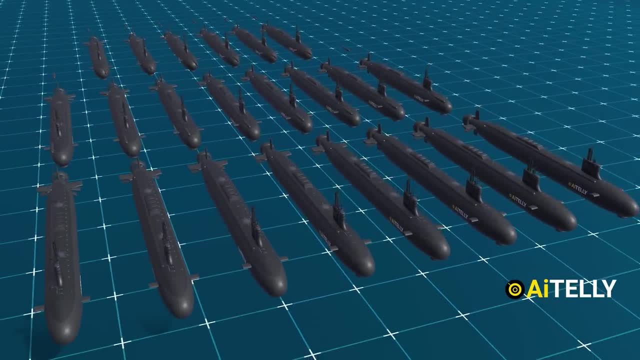 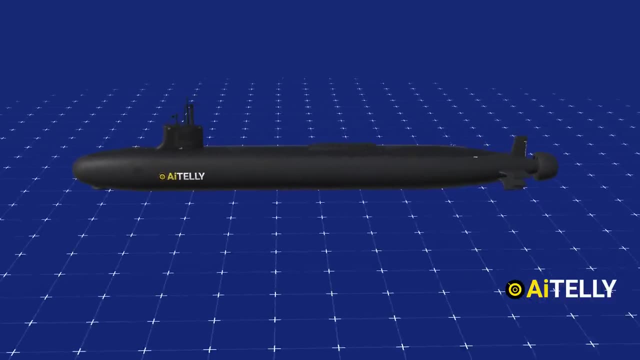 boats were planned to be built, but only 22 were completed. There are different versions of Virginia-class submarines, but let's take this as a base. The latest version, the Seawolf, commands a length of 460 feet or 140 meters, which is almost the length of four basketball courts. 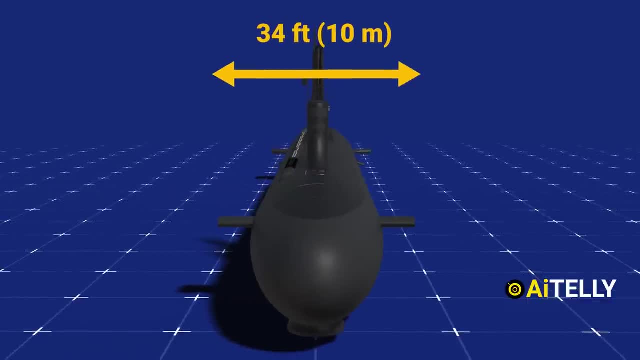 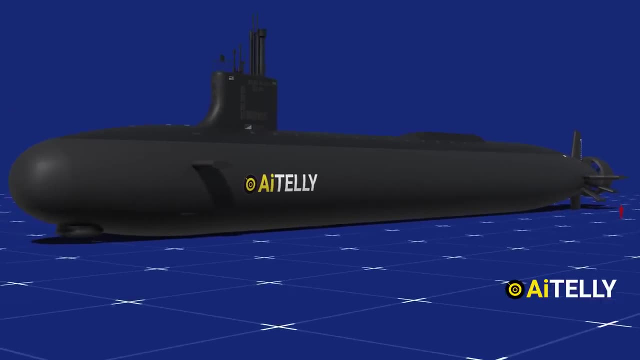 Interestingly, the beam is around 35 feet or 10 meters in height. Let's compare this to a person to help us visualize how huge this underwater beast is. Even better, to help us understand its volume, we found out: you can fit as many as 80 buses. 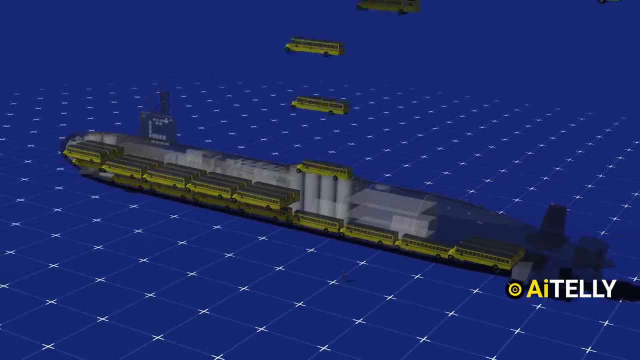 inside this submarine. if all are stacked one top of the other, That's a lot of school bus parking area for a nuclear-powered submarine. If all are stacked one top of the other, that's a lot of school bus parking area for a nuclear-powered submarine. 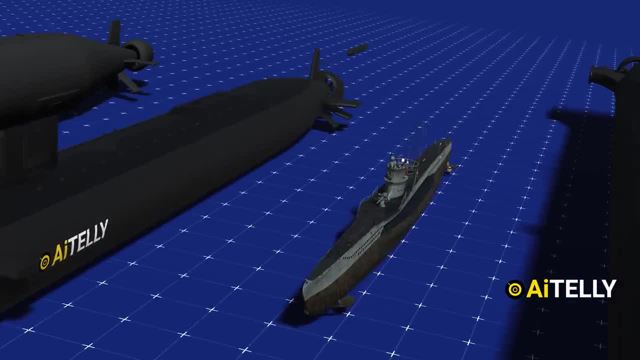 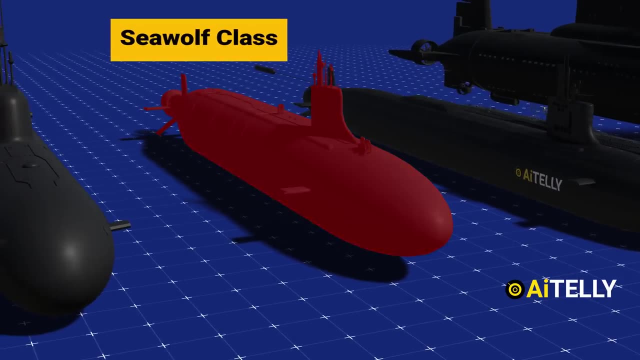 If all are stacked one top of the other, that's a lot of school bus parking area for a nuclear-powered submarine. Comparing it with different submarines, like this German U-boat built during WW2, it looks a lot smaller. This is the American nuclear Seawolf Fast Attack submarine. 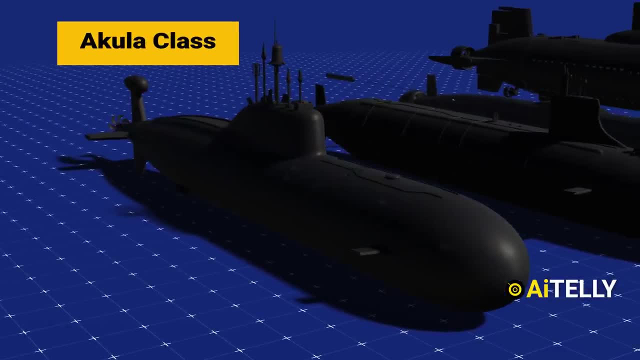 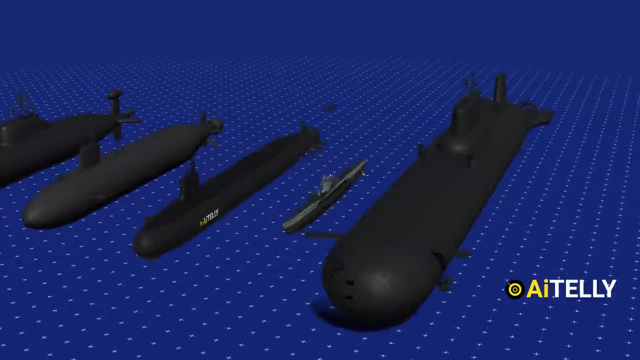 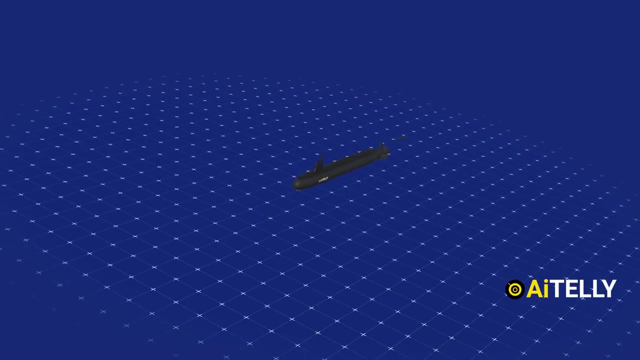 Beside it is the Russian Akula-class nuclear-powered submarine, And this last one is one of the biggest Russian Typhoon Class, also nuclear-powered, built during the Cold War era and still in service today. It weighs around 10,200 tons, which is almost the weight of 41 Air Force 1 planes. 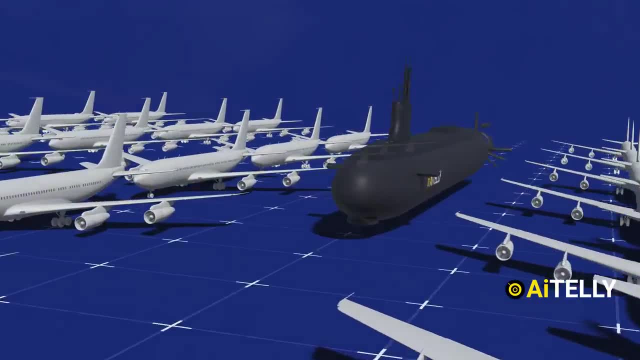 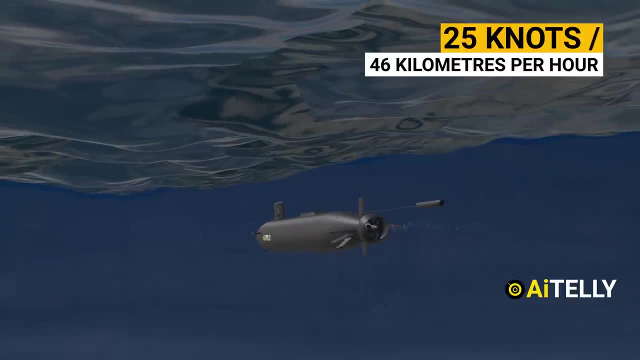 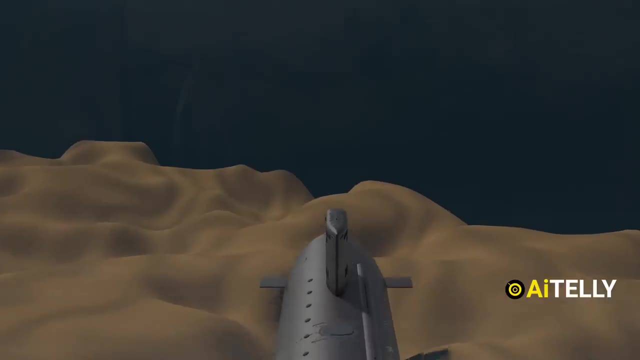 used by the president of america. that's a lot of weight on its shoulder. still, we should not underestimate its endurance, as it can command a speed of 25 knots or 46 kilometers per hour and over, and it can go to depths of 800 feet or 240 meters. this submarine range is unlimited, considering. 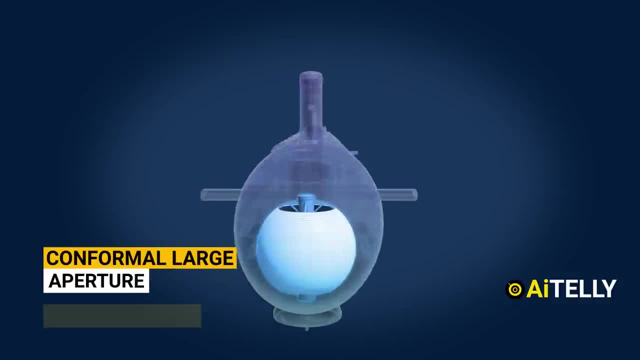 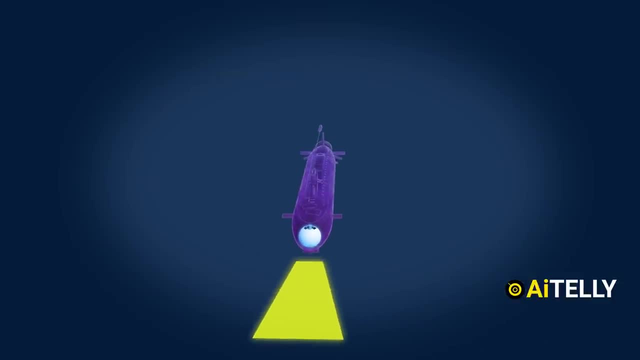 it is nuclear powered. this is the conformal large aperture sonar array, equipped with both active and passive versions of sonars. this is how it works. active sonar emits pulses of sound waves that travel through the water and reflect off the target and return to the ship by knowing the 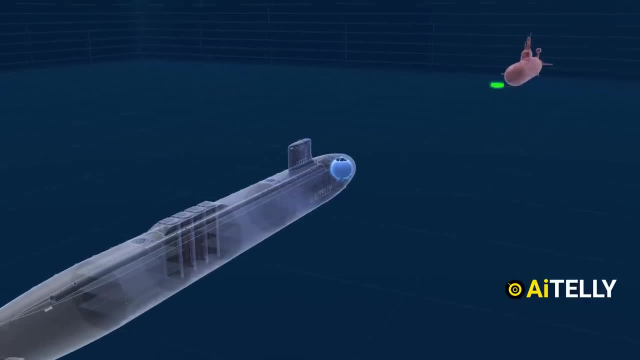 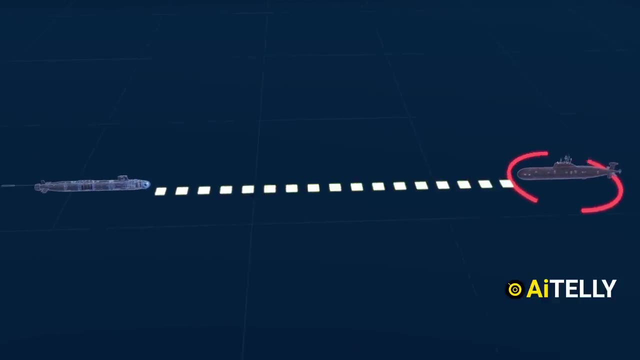 speed of sound and water and the time for the sound wave to travel to the target and back. the computers can then quickly calculate the distance between the submarine and the target in a short amount of time, but the virginia class uses an advanced passive sonar that maps the ocean. 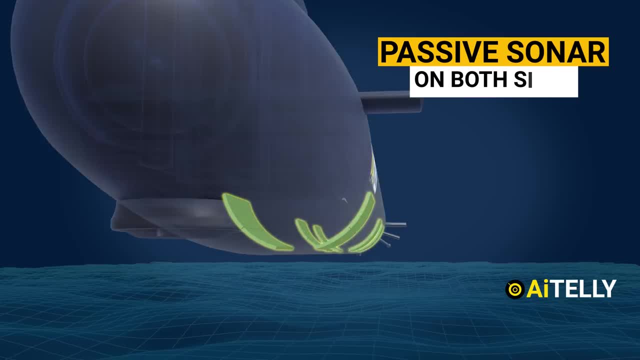 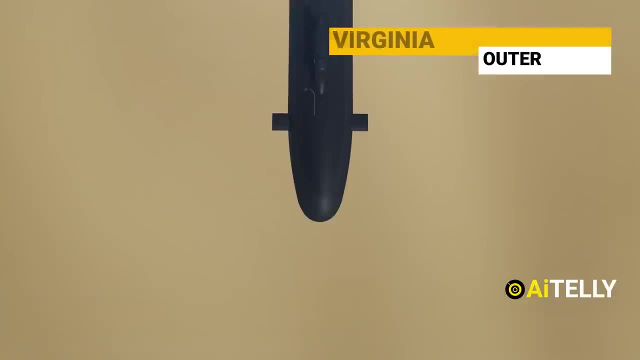 floors and minefields. additionally, you can also use the passive sonar to map the ocean floors and minefields. the sonar array are also attached on each side along with the long boom array to provide quick, target location and information. just behind the sonar section are the virginia payload tube outer. 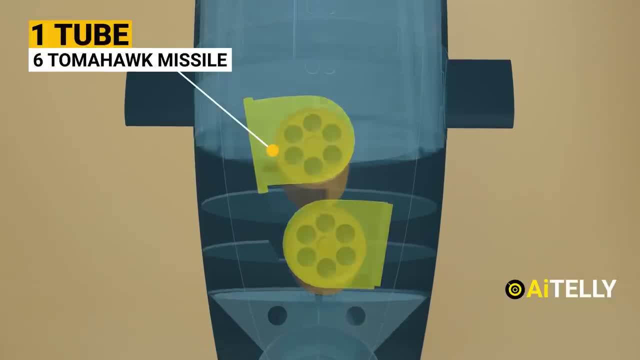 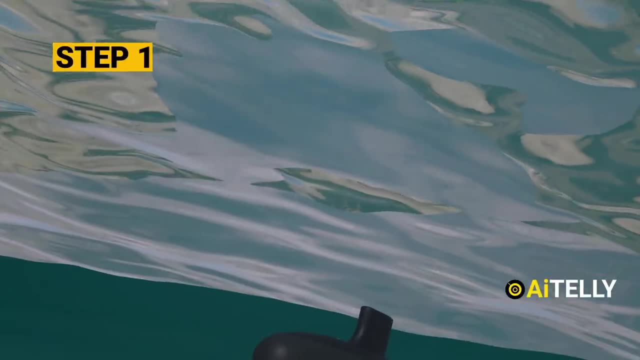 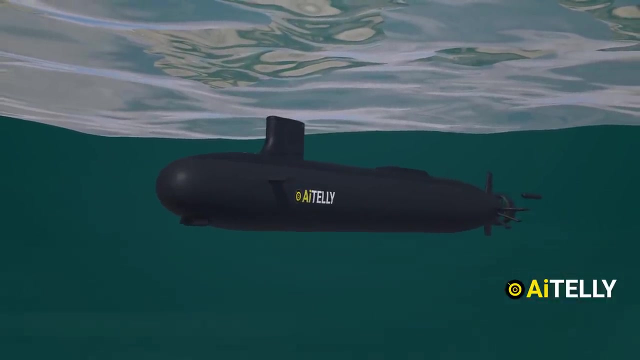 hatch. two of them can be found just besides each other. inside the tube are sixth kumamahawk missile. let's see how this works. step number one: a submarine will ascend to an assigned depth. step number two: when ready to launch, it will open up the hatch and the protective seal will break open. 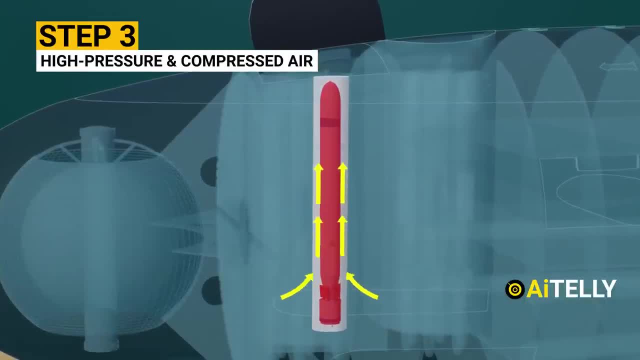 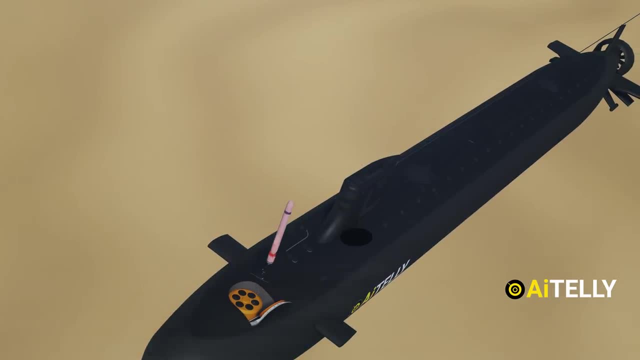 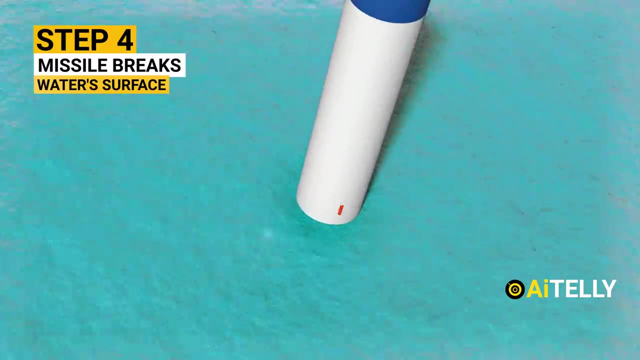 step number three: high pressure and compressed air is pumped into the tubes and this is used to eject the tomahawk missiles. step number four: the tip of the missile breaks the water's surface. step number five: the rocket boosters fire and propel the missile into its path. boosters fall off as soon as the missile is flat. 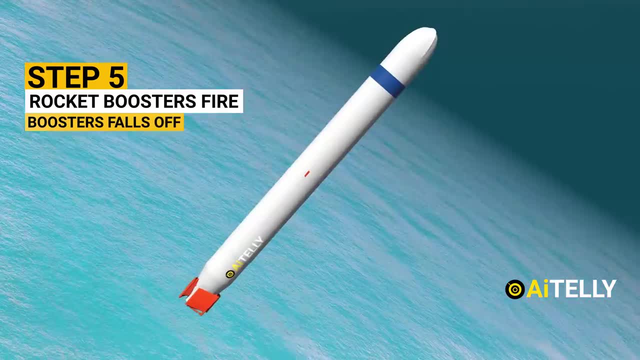 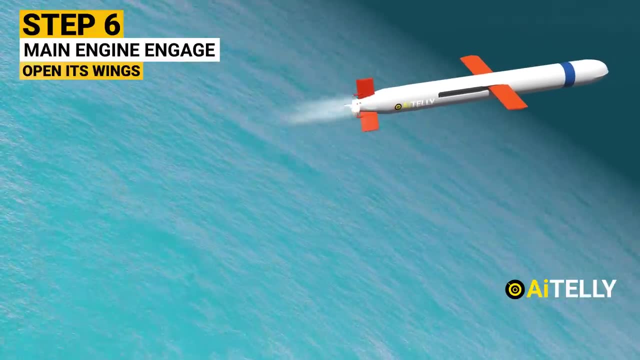 the rocket boosters fire and propel the missile into its path. boosters fall off as soon as the is out of the water. Step number six, The main engine of the Tomahawk missile, will engage and then it will open its wings, just like the animation shown here. 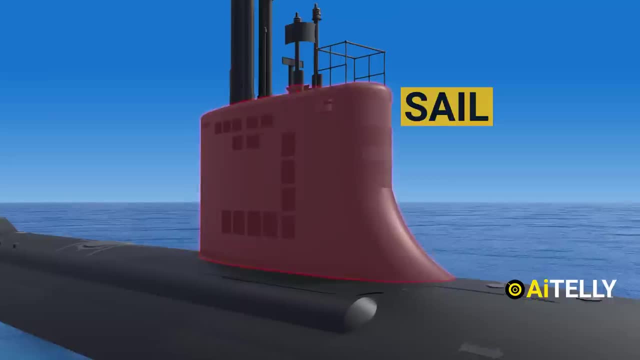 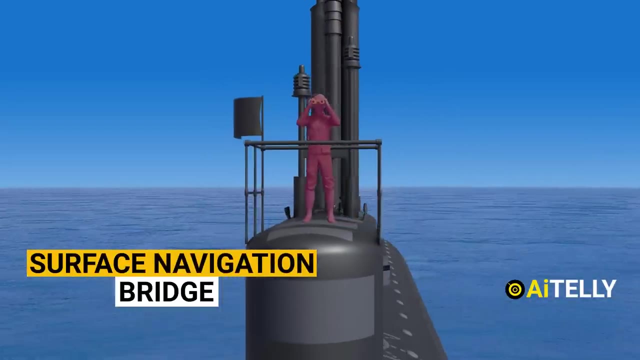 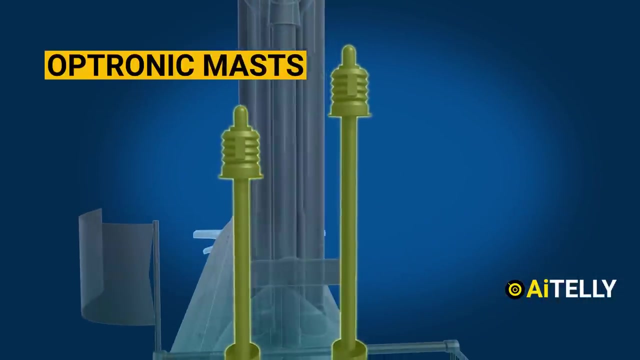 Moving ahead is the sail. for size visualization purposes, Let's compare this to the height of a sailor. This is the surface navigation bridge, where sailors or commanders stand on top for outside observation. These are the two octronic masts, a sensor on a submarine that functions similarly to 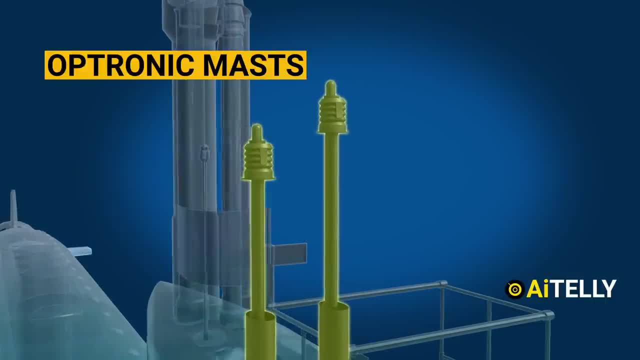 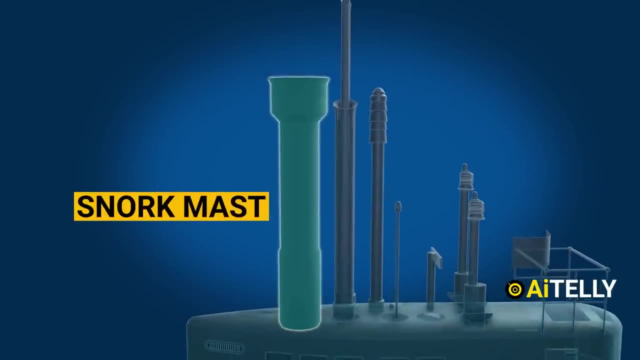 a periscope without requiring a mechanical tube Moving ahead. this is the communication mast required to send and receive data. At the back is the snort mast. Snorkel is a device which allows a submarine to operate submerged while still taking in. 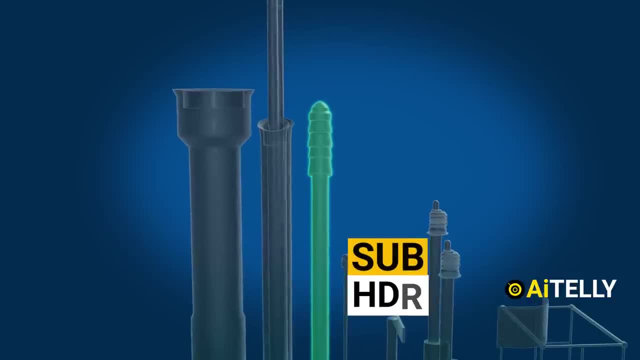 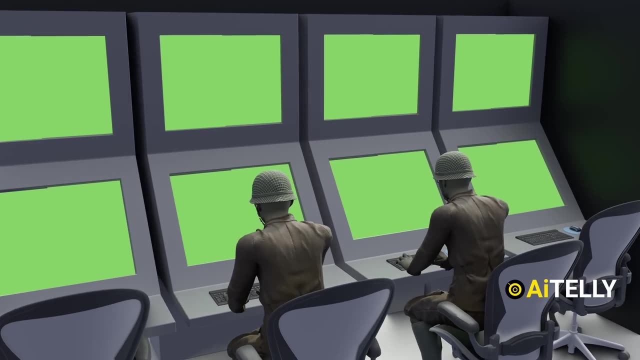 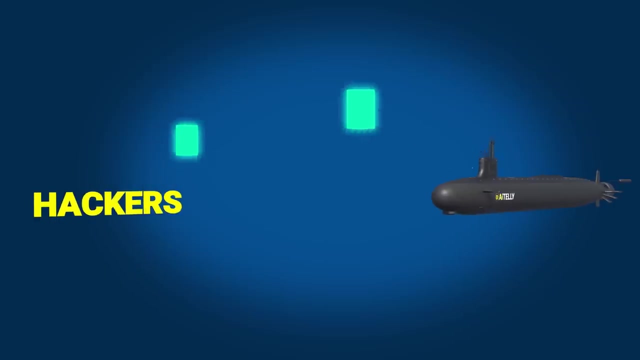 air from above the surface. This is the sub-HDR high data rate satellite communication. But just a reminder: this is no ordinary internet connection and has a military grade data encryption level for using the internet, because you do not want hackers. If you are a civilian, you can also use this level of encryption by using private internet. 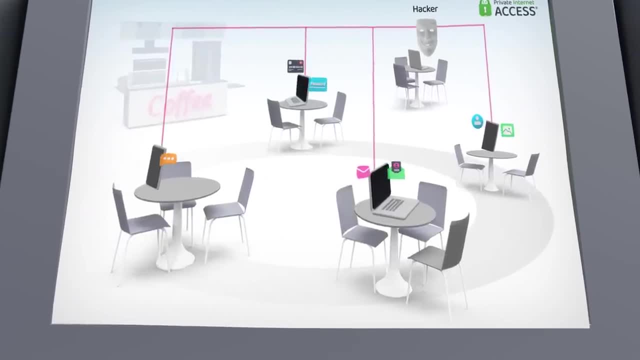 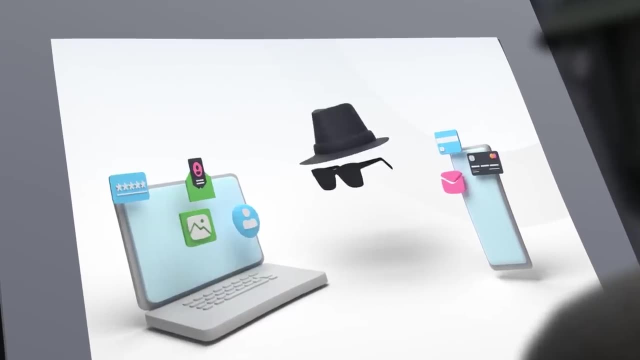 access. Whenever you are browsing online on an unprotected device such as your phone, computer, tablet or console, your device is transmitting a great amount of information out into the open, which can be viewed by various different entities before reaching the intended website. 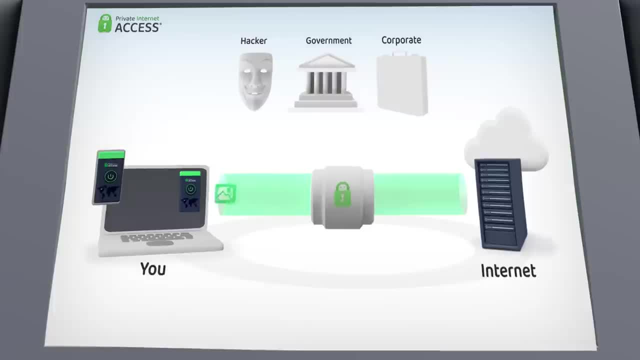 A virtual private network- or VPN for short, hides your IP address and safeguards your internet connection through the internet. Step number seven: If you are a civilian, you can also use the unprotected internet connection. If you are a civilian, you can also use the unprotected internet connection through an. 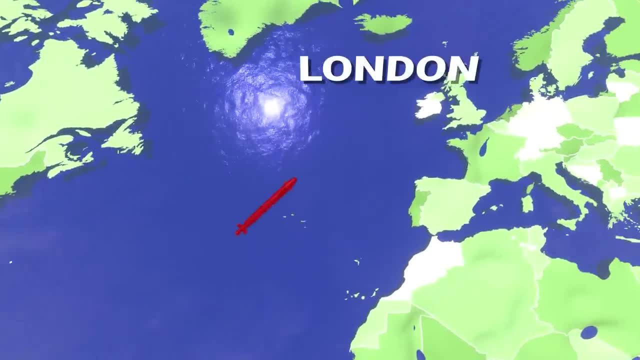 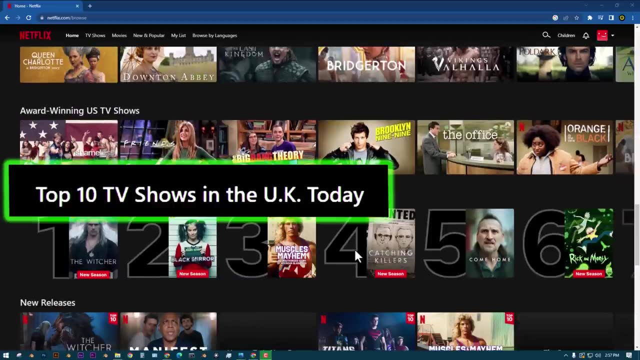 encrypted tunnel. Taking this guy as a reference, as he is sailing from America to London, His websites and services across the internet will change and accessible depending on his physical location. Here is my account. As you can see, I am in the UK version of Netflix. 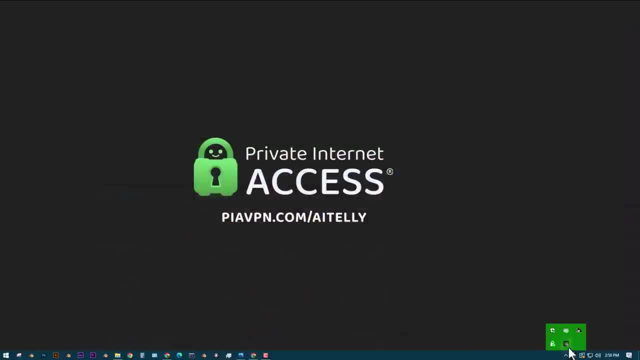 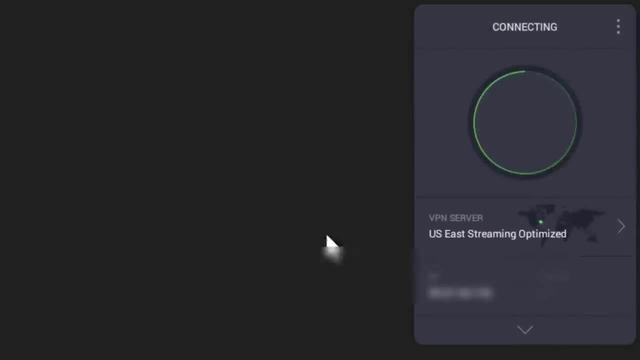 To switch to a US server, I just use Private Internet Access VPN. This is a London server- and to switch to a different server, I just have to scroll here and select US Streaming Optimized Server, which is going to be used for streaming content specifically. 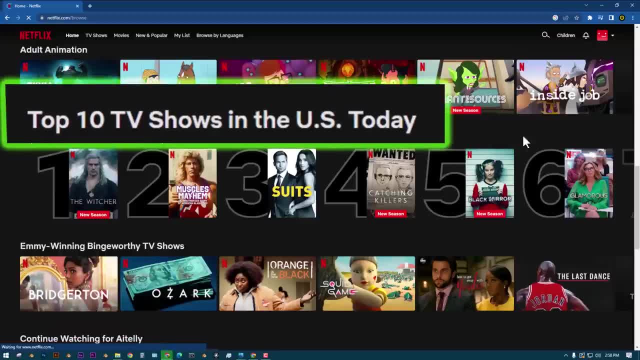 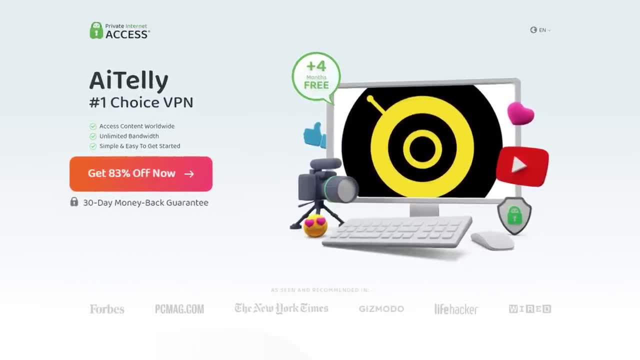 Then go to our web browser, refresh it and boom, here we go- Netflix US region. But wait, that's not it. You can now use one Private Internet Access subscription to protect an unlimited amount of devices at the same time, just for the price of one account. Go to piavpncom, slash ai-tele for an 83% discount on Private Internet Access. That's $2.03 a month and get four extra months for free. That's $2.03 a month and get four extra months for free. 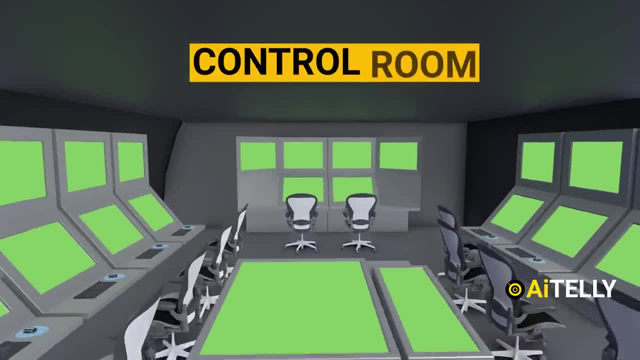 That's $2.03 a month and get four extra months for free. That's $2.10 a month and get 6 international tickets today And that will be $ revelation and 54% off. This is the control room and it is divided into various sections. 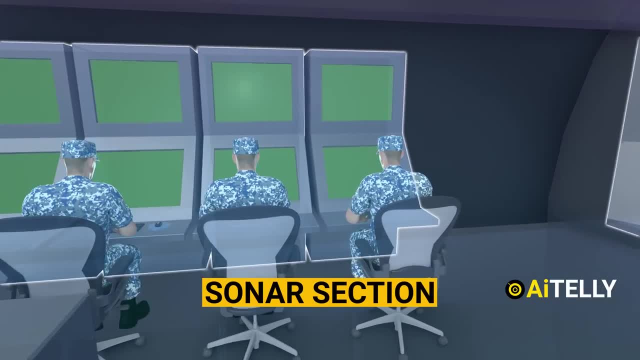 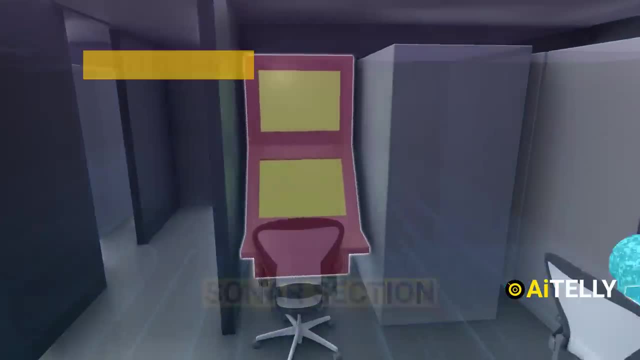 This is the ship control department. Interestingly, the sonar section has the highest number of technicians working on it, as they are the eyes and ears beneath and above the ocean. This is the photonics and navigation department is by Office developer, which is digitally. 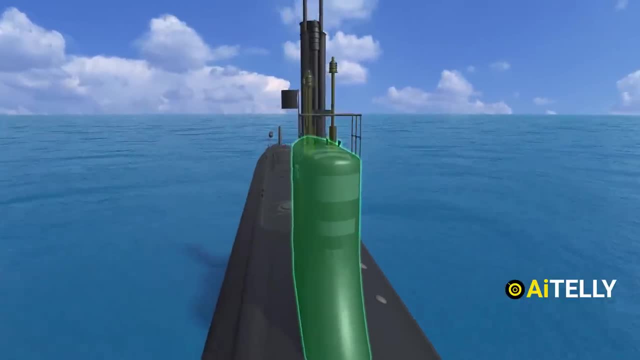 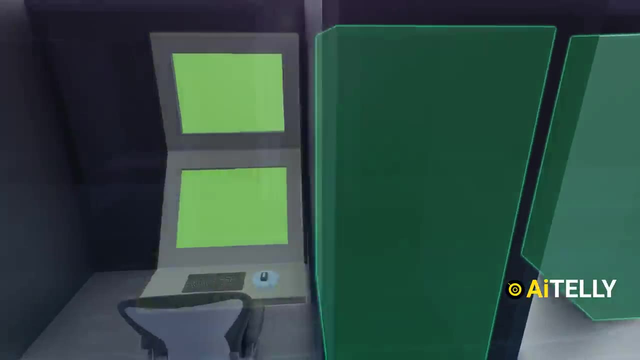 linked to the sail and it can also be described as the modern age periscope known as the photonics. Here lies the radio room, 4TH BATHERN APLICATION ESSENTIAL INSTALLATION. beside it is the special operation room and the last section is the combat and control room that 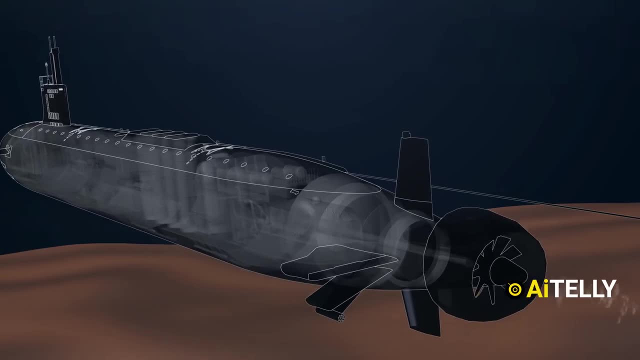 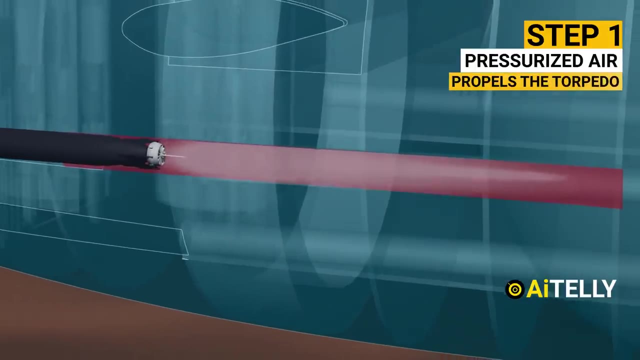 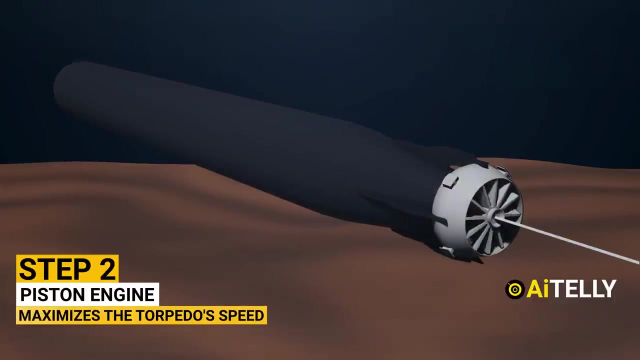 fires the missiles as well as the torpedo. This is how a torpedo works, explained in very basic animation. Step number one: Pressurized air propels the torpedo toward its target. Step number two: A piston engine with propellers maximizes the torpedo's speed. Step number three: It trails a. 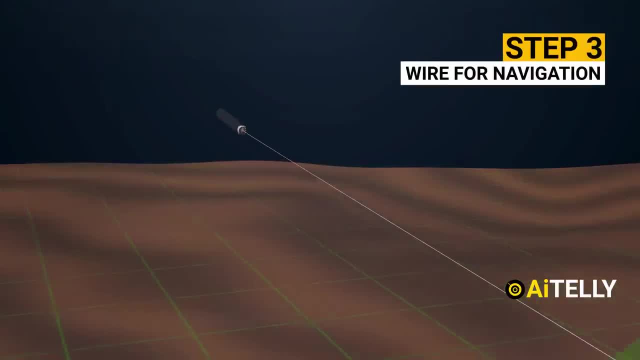 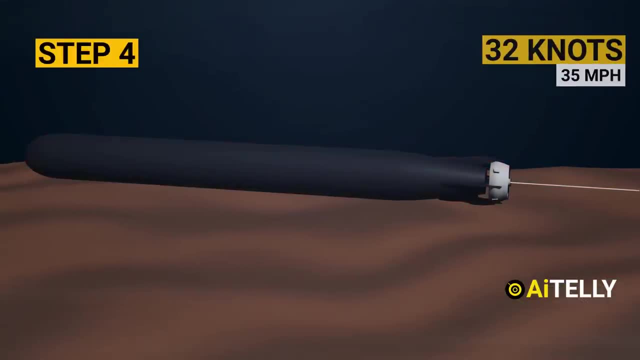 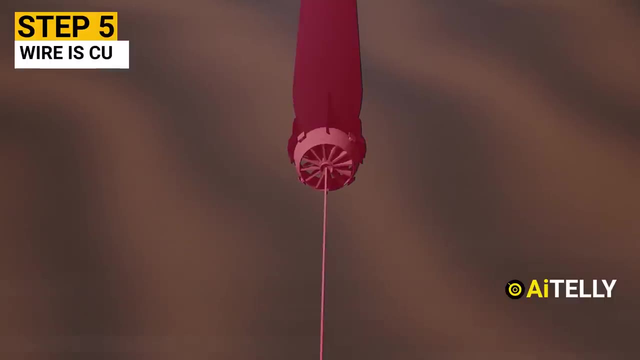 wire plugged into the weapons systems aboard the sub, using data to navigate. Step number four: The torpedo accelerates to 32 knots, over 35 miles an hour, with a range of 8 miles or 12 kilometers. Step number five: As it nears its target, the wire is cut and its sonar takes over navigation. 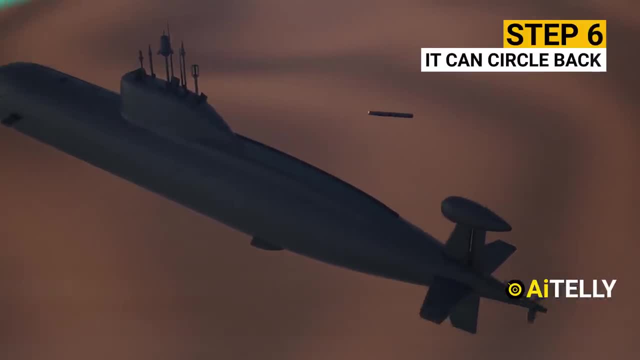 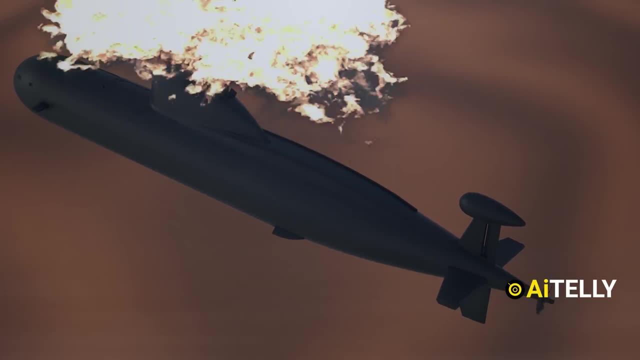 Step number six: If a torpedo misses its target, it can circle back and starts hunting the target with its sonar. This one torpedo has the explosive power of 1200 pounds of TNT and I guess you do not want to be at the receiving end of this weapon. 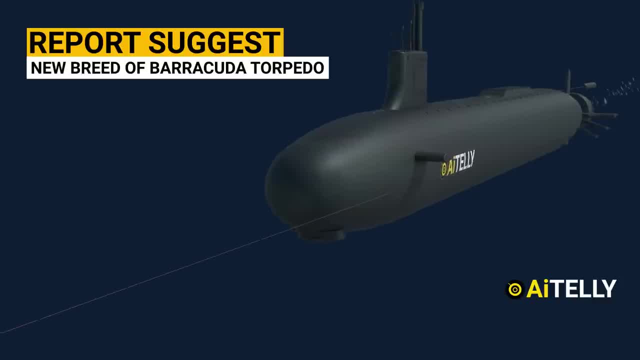 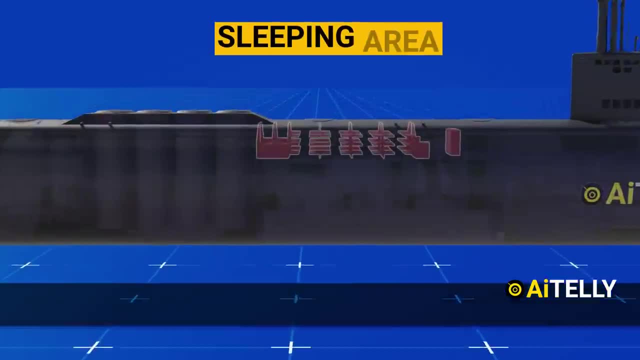 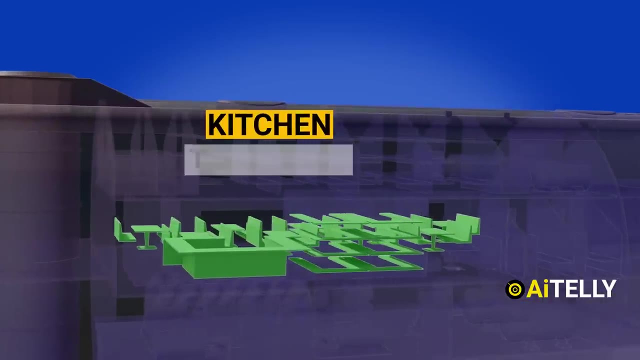 but reports suggest that new breed of barricaded torpedo or super cavitating are going to be the latest upgrades. This upper section is the sleeping area of the crew. It has around 119 permanent berths. Just below it is the kitchen, or some call this the galley. It also has a ward room. in simple, 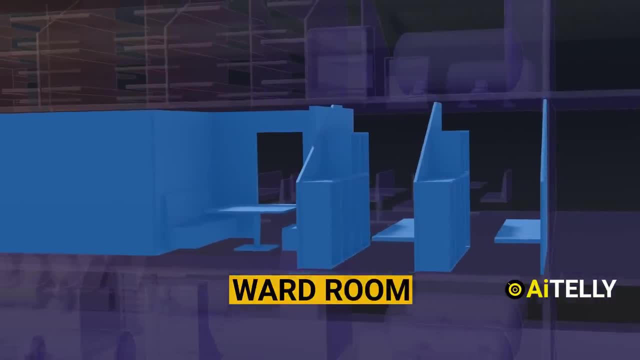 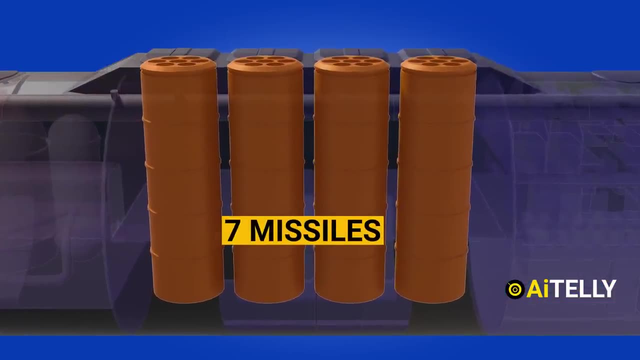 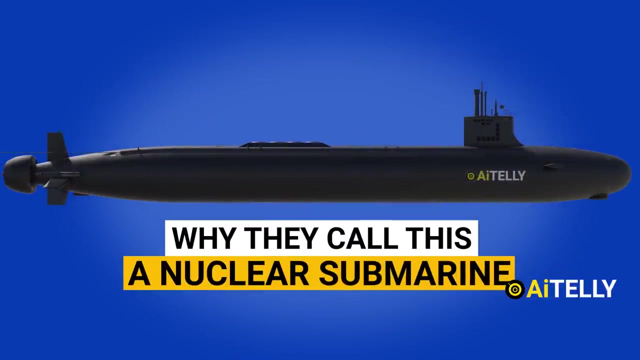 words. it's a section where sailors eat lunch, dinner or conduct mission meetings. Moving to the back is the uprated Virginia modules, which can hold around seven missiles, That is, around 28 missiles just with these four tubes. and now the most important part is why they call this a nuclear submarine. Nuclear physics is a complicated 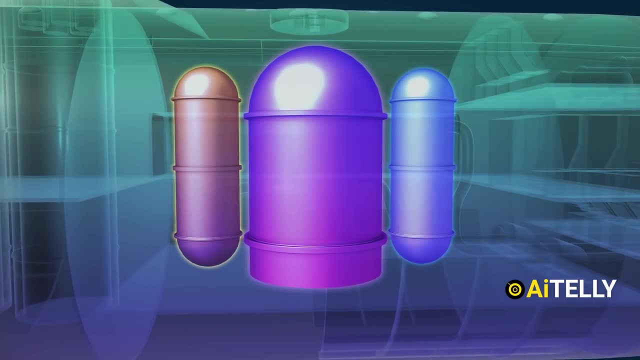 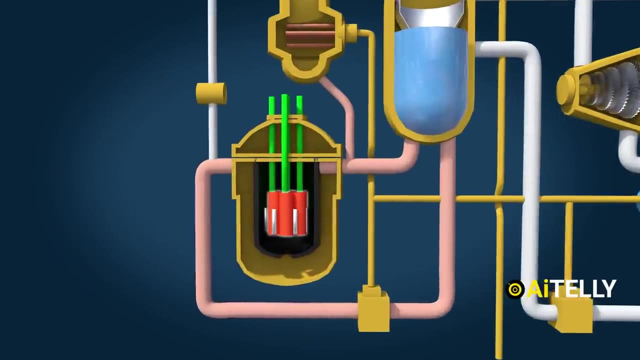 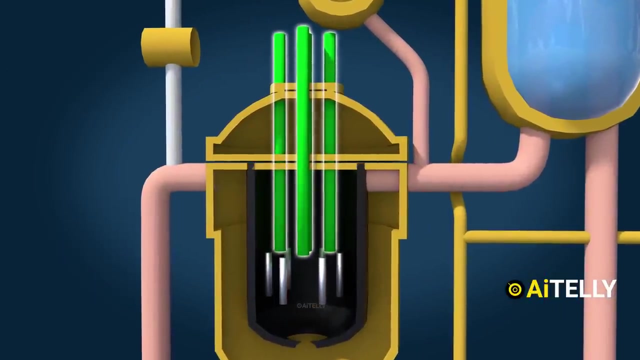 subject, but we will try to explain the basic process in super simplified animation. as shown below, A nuclear reactor consists of three crucial components. One: fuel elements could be uranium-2,3,, 5 or uranium-2,3,8, and these rods vary in number according to the size of the reactor. Two: 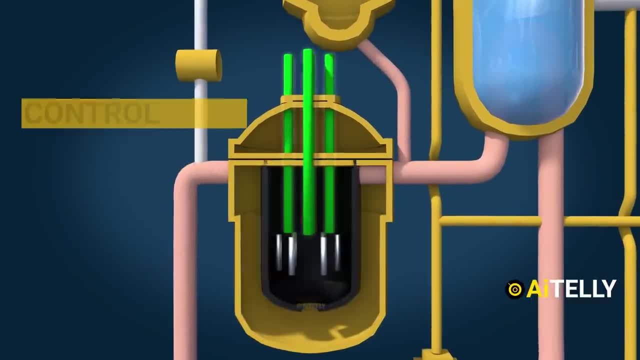 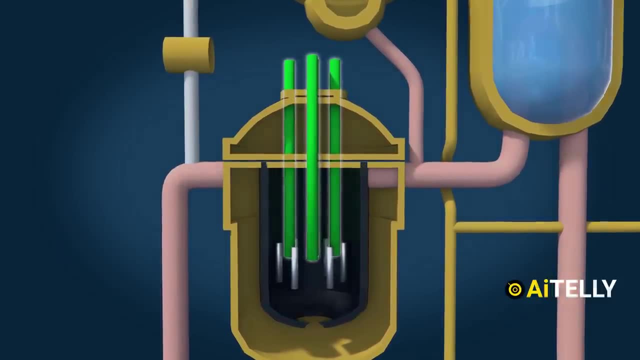 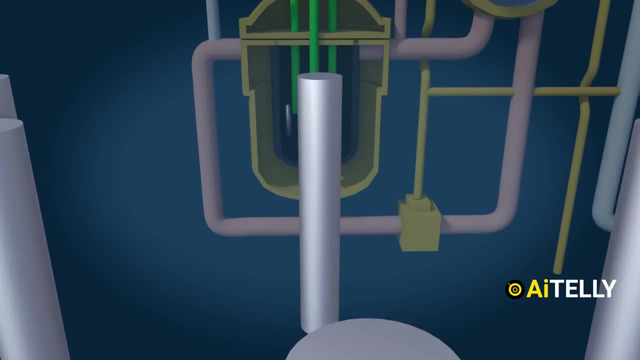 moderator here can be water Three. these are the control rods and the main function is to absorb any excess or spare neutron in the moderator. that is water. Let's see how it works: Uranium oxide is compressed into fuel. Parts of uranium are packed into sealed fuel rods. The fission of the 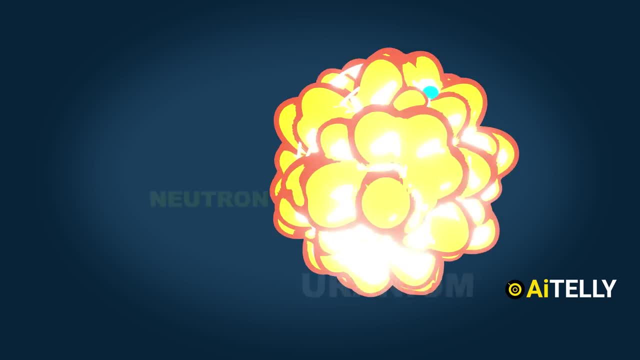 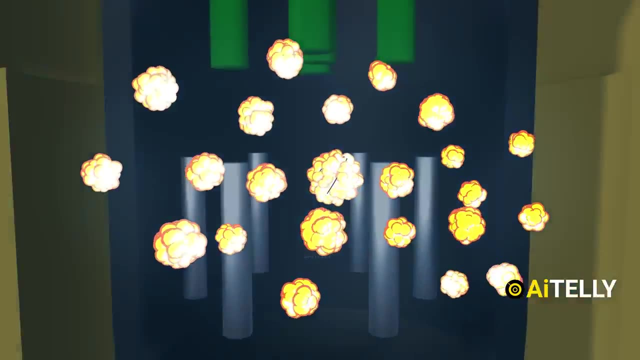 uranium begins by bombarding the reactor with fuel. The fission of the uranium begins by bombarding it with neutrons. In each fission, two or three neutrons are released. This in turn cause new fission and thus creating a chain reaction. But in a nuclear reactor it's important that this chain 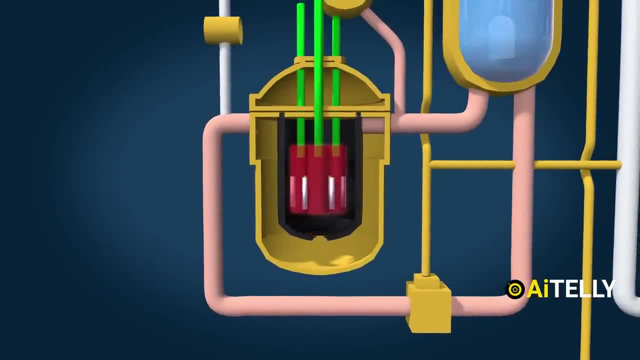 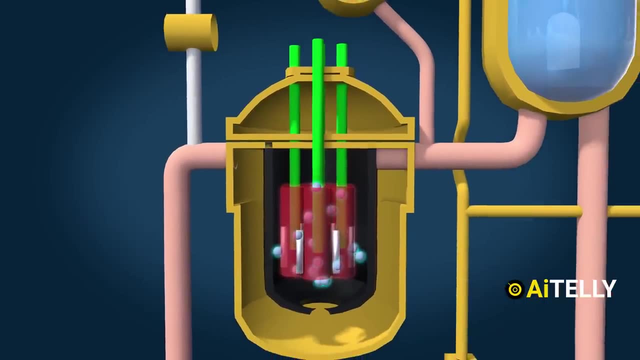 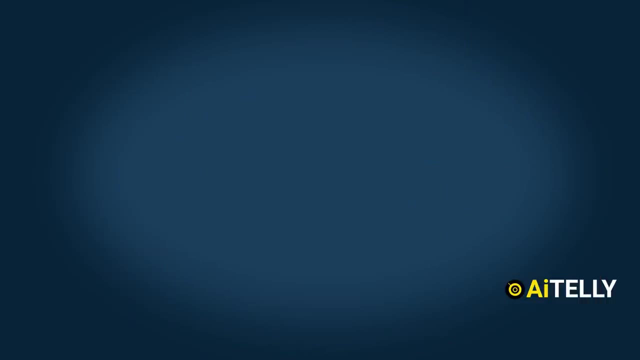 reaction is controlled. after each fission, Only one released neutron should cause new fission. This is how it is controlled: By lowering the control rods. it absorbs the oversupply of neutrons, Lowering all the control rods at the same time, and the result is it helps stop the chain reaction Now. 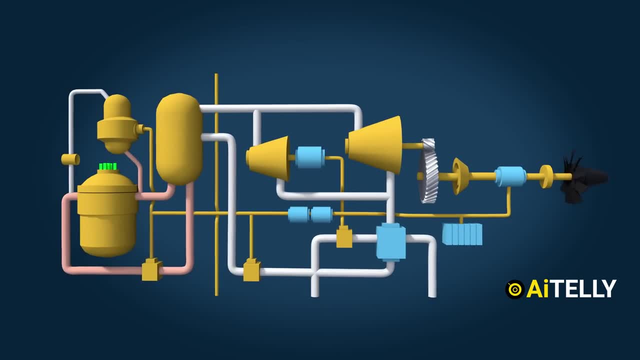 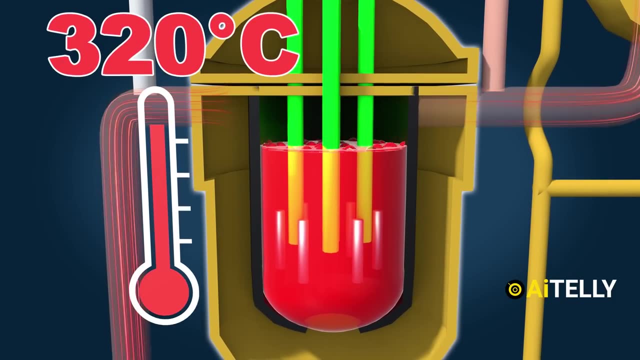 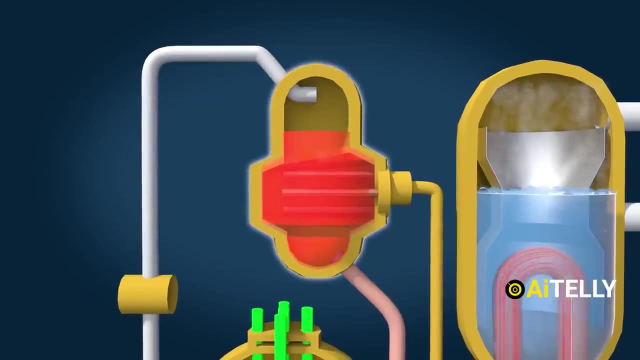 that we have mastered the basic understanding of a nuclear reactor, let's look at the step-by-step process. Step number one: the nuclear reactors heats the water to 320 degrees Celsius. Step number two: his pressure regulator is responsible for preventing water from converting into steam. 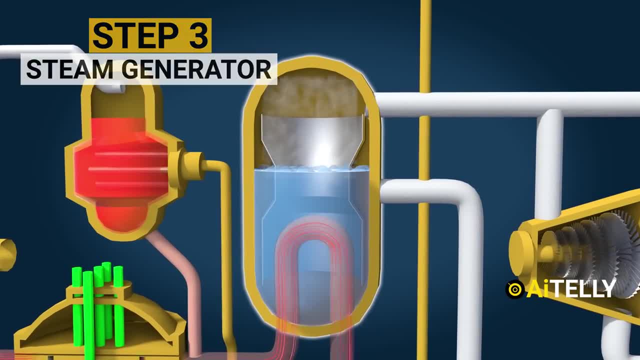 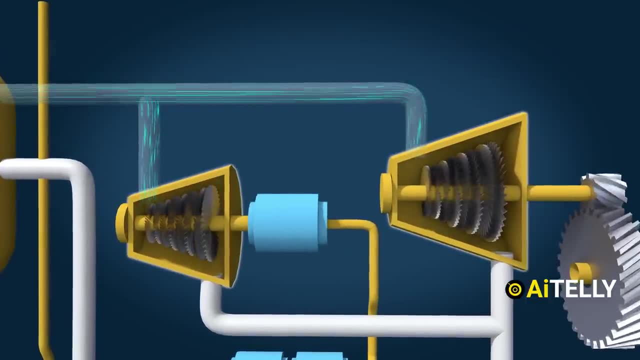 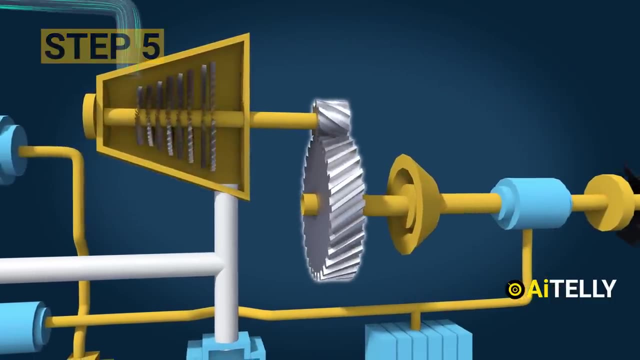 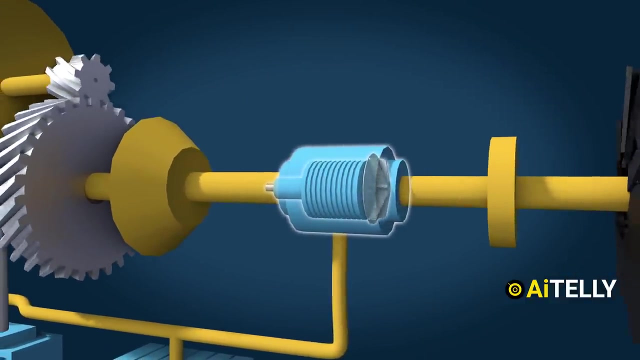 Step number three: high pressure passes through a steam generator. This is where you want to convert water into high pressure steam. Step number four: the steam generator helps turns these huge turbines at a very high speed. Step number five: the spinning turbines are connected to these gears. Step number six: the gears and clutch empowers the. 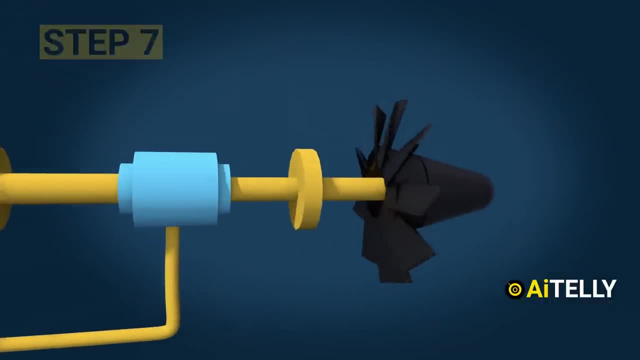 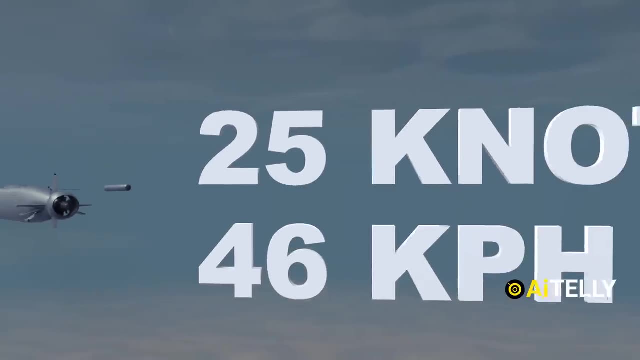 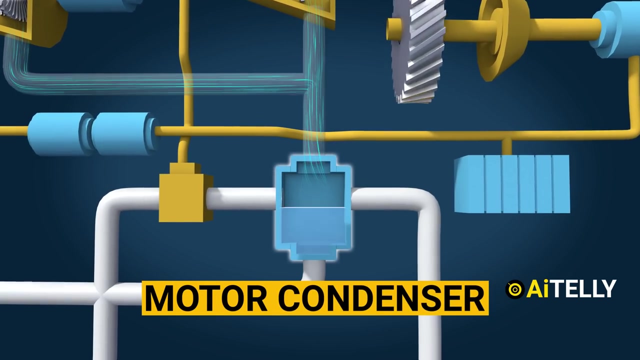 electric motor. Step number seven: this in turn powers the propellers of this huge underwater beast propelling at speeds of 25 knots or 46 kilometers per hour. Step number eight: the steam is then passed through a motor condenser, which turns into water. It is then pumped back into the 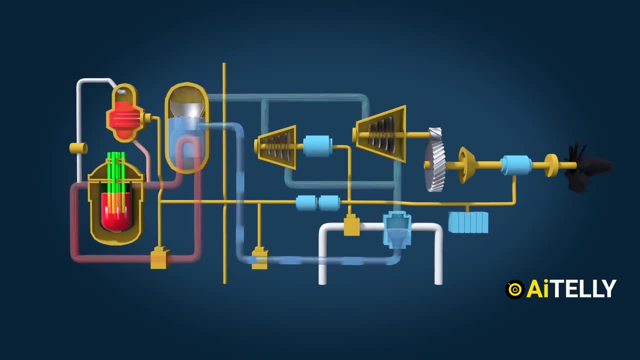 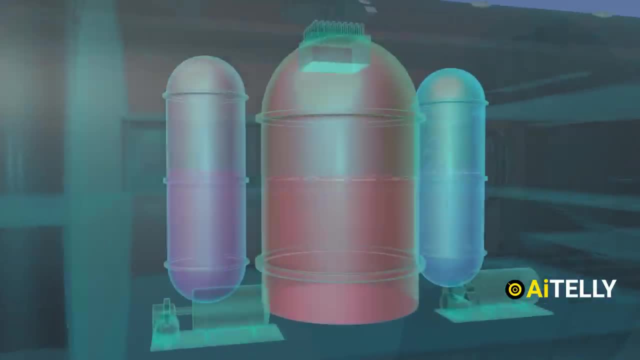 steam generator and the process is repeated, giving it almost an unlimited fuel for the submarine. Now that you have understood the basic of a nuclear reactor, this is how it works in a Virginia-class nuclear submarine. The heat for this nuclear reactor is used to generate steam. 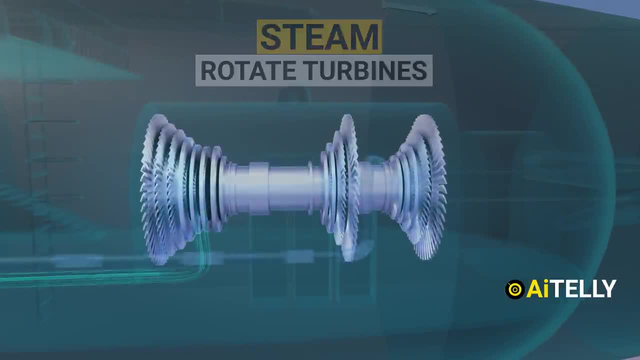 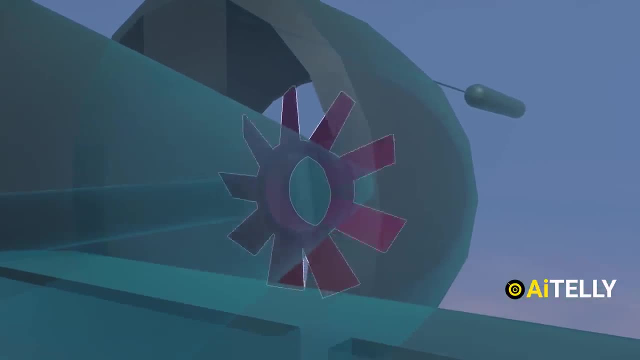 This steam is then used to rotate a series of turbines, forcing the blades to turn at a high speed. In a more simplified animation, the steam is then pumped back into the steam generator and the propellers are then propelled back into the steam generator. In a more simplified animation, 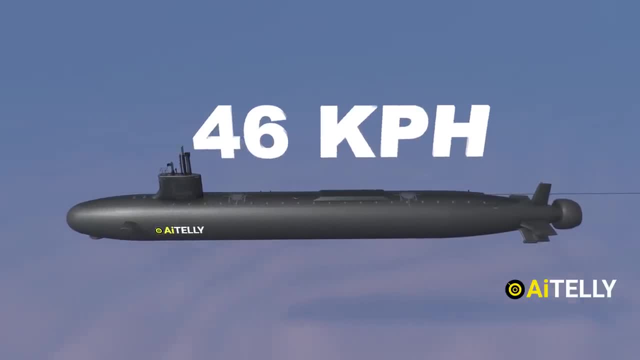 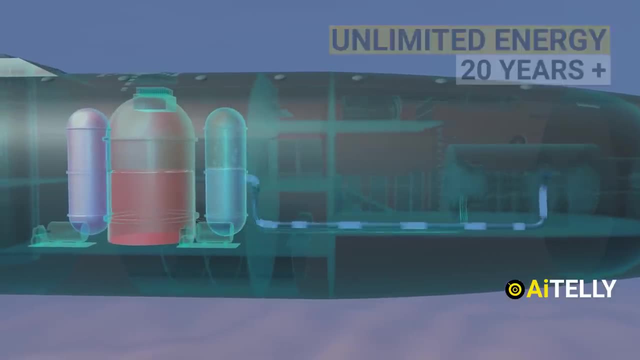 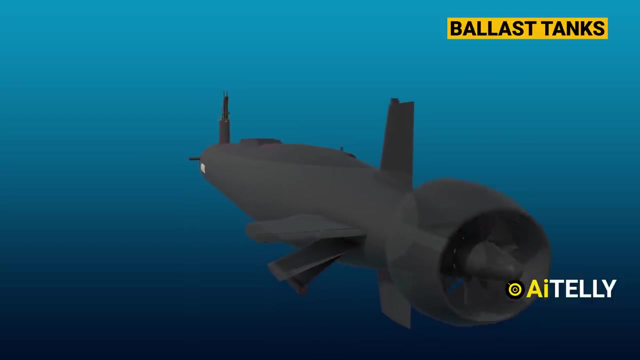 these then drove the propellers, moving this 10,200 tons underwater beast at a speed of 46 kilometers per hour or 28 miles per hour. This is unlimited energy of about 20 years without needing to refuel and only limited by the sailor's food supply Ballast tank technology. 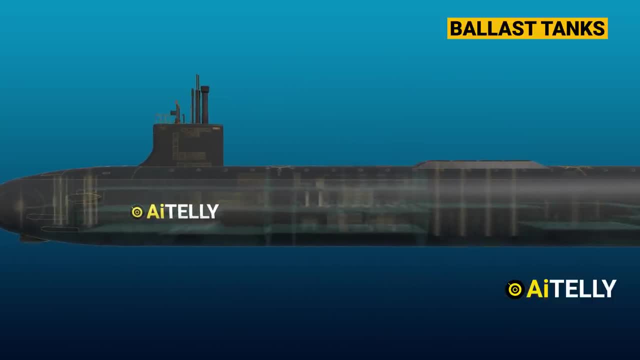 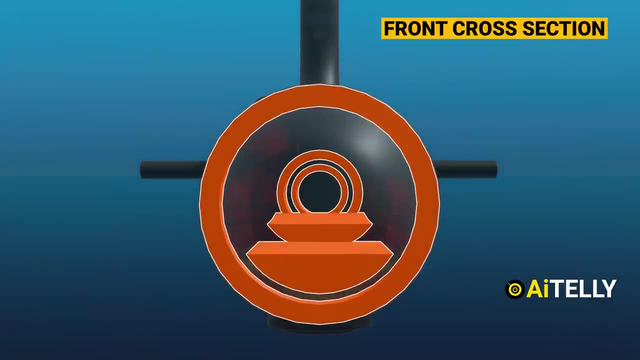 is a complicated process, but we will present it to you in a super simplified animation. In a submarine there are ballast tanks attached to both the front and back and even in the middle. The tanks have flood ports at the bottom and valves at the top.